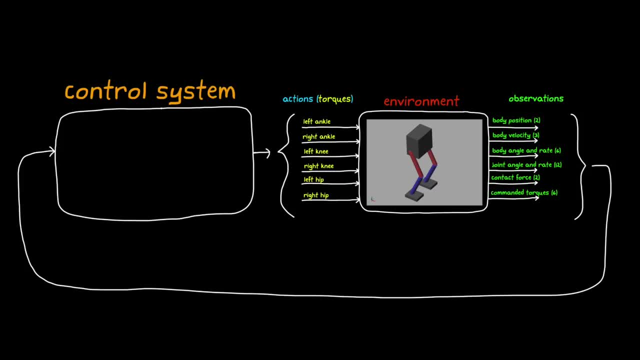 to be for even this really simple system. Now, as I mentioned in previous videos, rather than try to design the logic, the loops, the controllers, the parameters and all that stuff using the traditional tools of control theory, we can replace this whole massive function end-to-end with a. 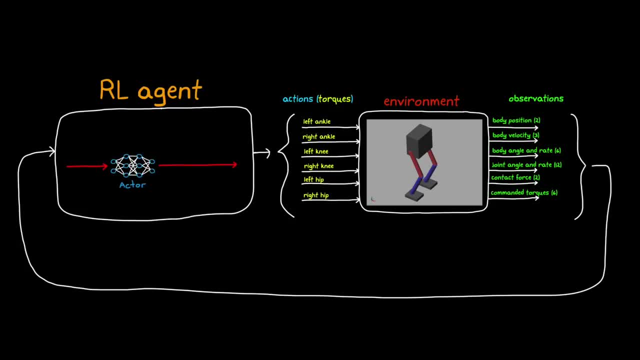 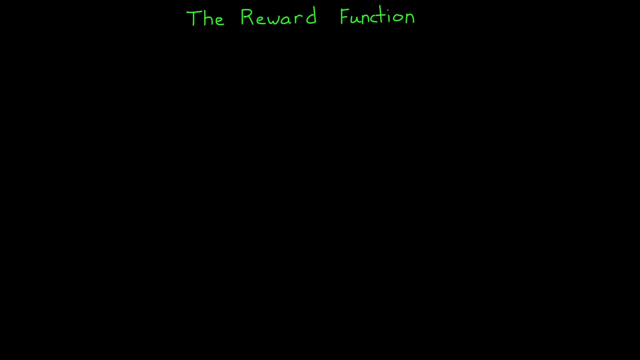 reinforcement layer. So what we're going to do here is we're going to use an agent learning agent, one that uses an actor network to map these 31 observations to the six actions, and a critic network to make the training more efficient. As we know, the training process requires a reward function, something that 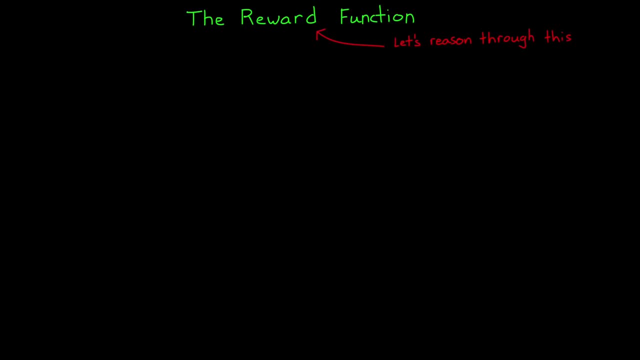 tells the agent how it's doing so that it can learn from its actions, And I want to reason through what should exist in the reward function by thinking about the conditions that are important for a walking robot. This might be how you'd approach building up a reward function, if you. 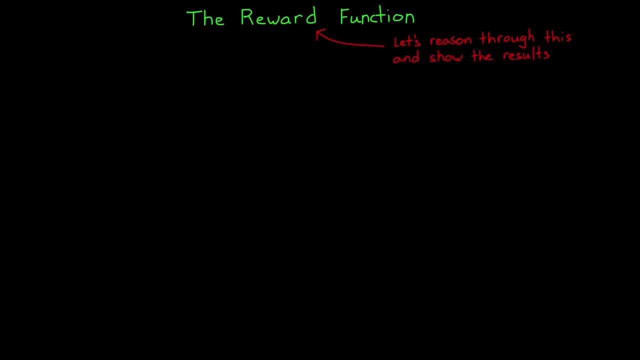 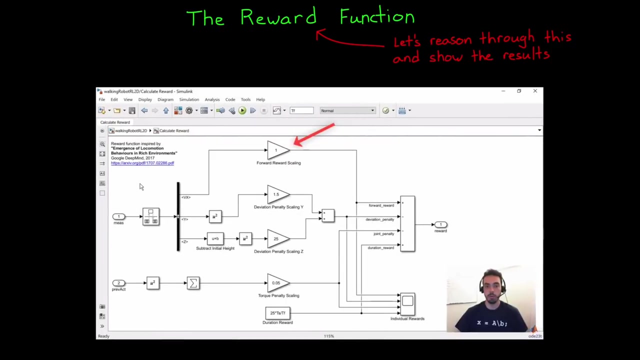 want to, So I'm going to show you the results of training with this function as we create it, so you can see how the changes impact the solution. However, I'm not going to go over how to run the model, because there's already a great video by Sebastian Castro that does just. 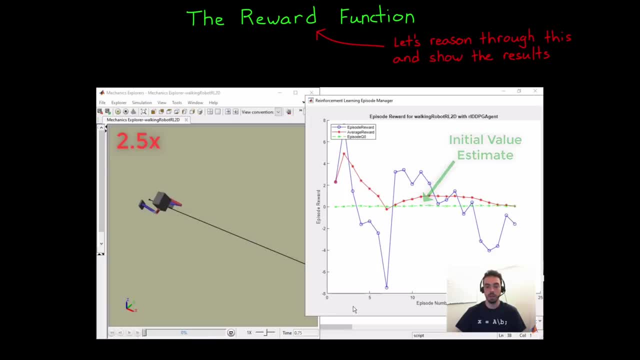 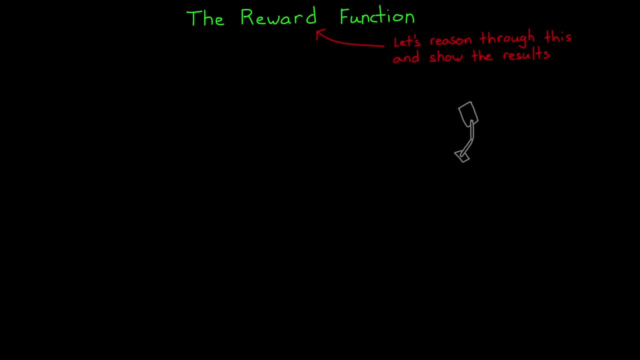 that. So if you're interested in trying out all of this on your own, I'd recommend checking out the link in the description below. All right, so on to the reward. Where to start? We obviously want the body of the robot to move forward, otherwise it's just going to stand there. 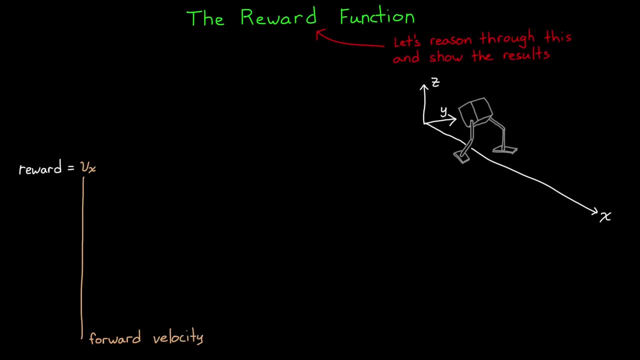 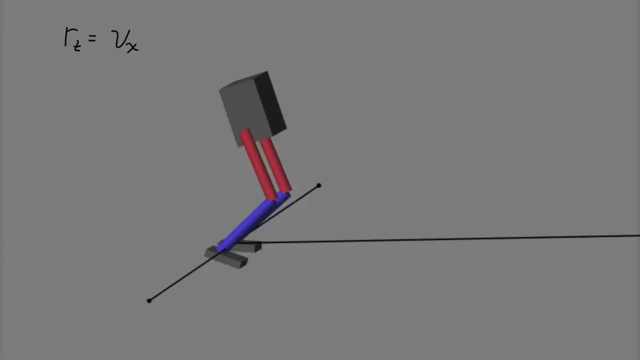 But instead of distance we can reward it for its forward velocity. That way there's a desire for the robot to walk faster rather than slower. In training, with this reward we can see that the robot dives forward to get that quick burst of speed at the beginning, and then it falls over. 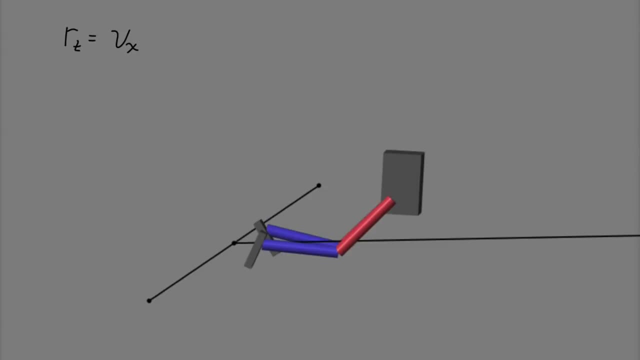 and doesn't really make it anywhere. Now it may eventually figure out how to make it further with this reward, but it was taking a long time to converge and not making a whole lot of progress. So let's think about what we can add to the reward. 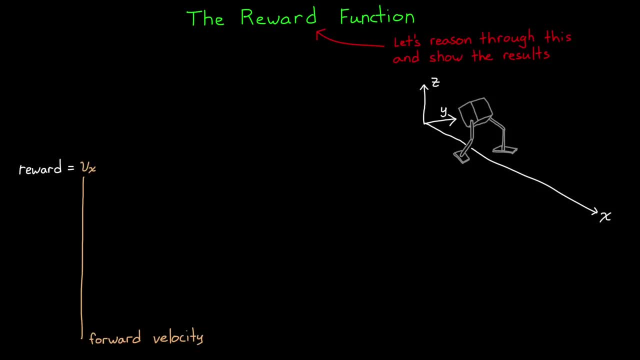 So we could penalize the robot for falling down so that it, when diving forward, isn't as attractive. So if it stays on its feet for a longer time, or if more sample times elapse before the simulation ends, then the agent should get more reward. Let's see how this one does. 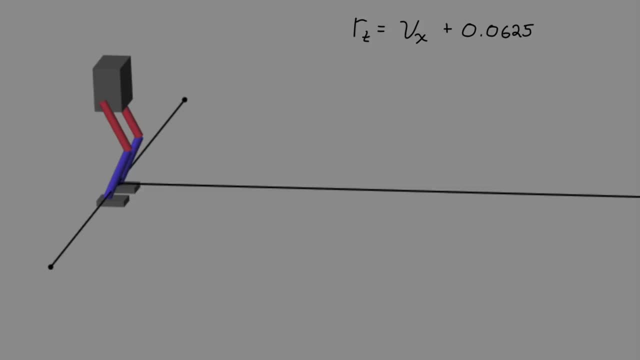 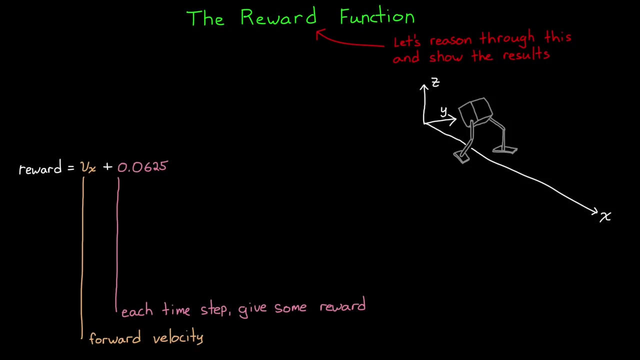 It's gotten a bit of a hop at the beginning before ultimately falling down. Perhaps if I'd let this agent train longer, I could have had a robot that jumps across the world like a frog, Which is cool, but not what I'm going for. So it's not enough that the robot moves forward and doesn't fall. 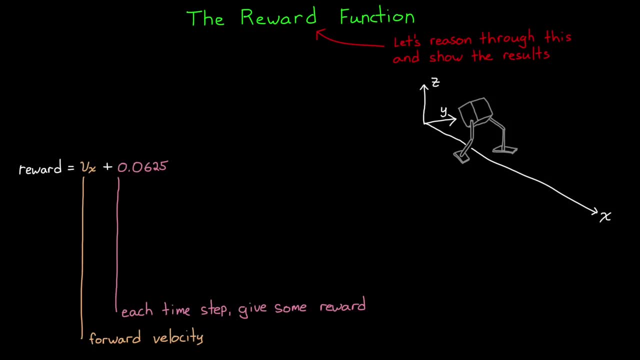 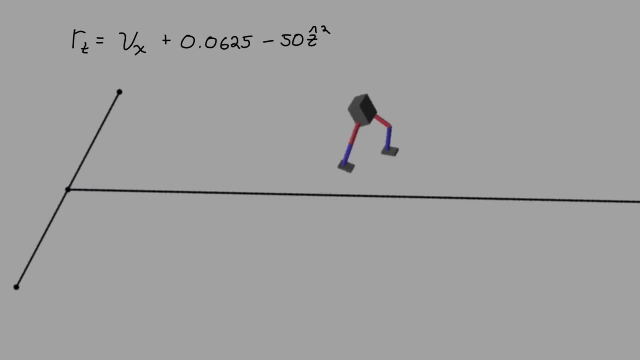 we want some semblance of walking instead of hopping or crouch walking. So to fix this, we should also reward the agent for keeping the body as close to a standing height as possible. Let's check out this reward function. Okay, this one's looking better, but the solution isn't really natural looking. It stops occasionally. 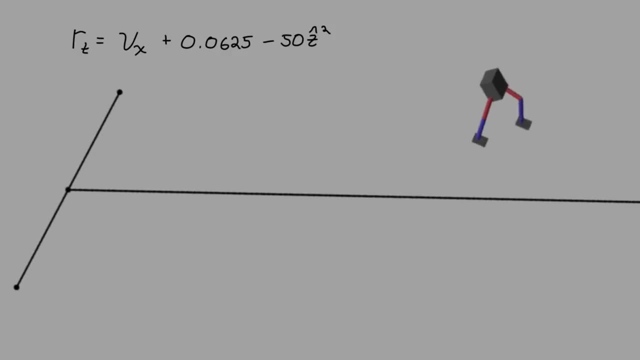 to sort of jitter its legs back and forth and most of the time it's dragging its right leg like a zombie and putting all of the actuation into the left leg, And this isn't ideal if we're concerned with actuator wear and tear or the amount of energy it takes to run this robot. We'd like 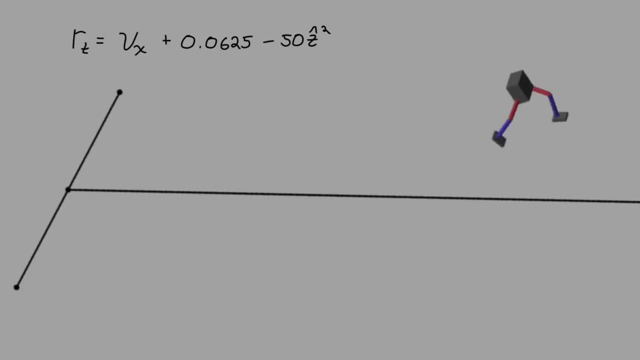 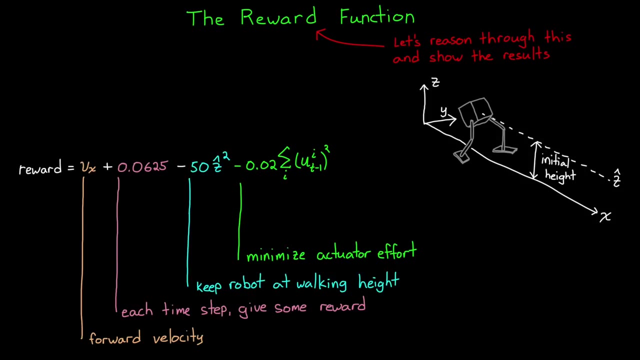 both legs to do equal work and not to overuse the actuators with a lot of jittering. So to fix this we can reward the agent for minimizing actuator effort. This should reduce extra jittering and balance the effort so that each leg has a share of the load. 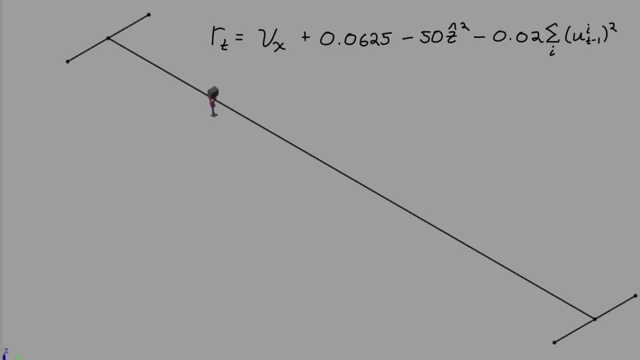 Let's check out this trained agent. Okay, we're getting really close here. This is looking pretty good, Except now we have one final problem. We want to keep the robot moving in a straight line and not veering off to the right or to the left like it's doing here. 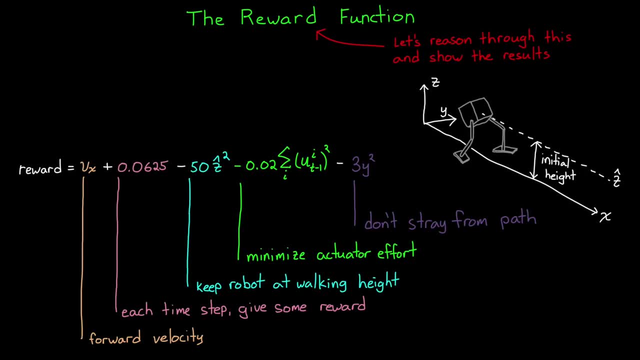 We want to reward it for staying close to the x-axis. This is our final reward, and training with it needs about 3500 simulations. So if we set this up in our model and we unleash the simulation on a computer with multiple cores, 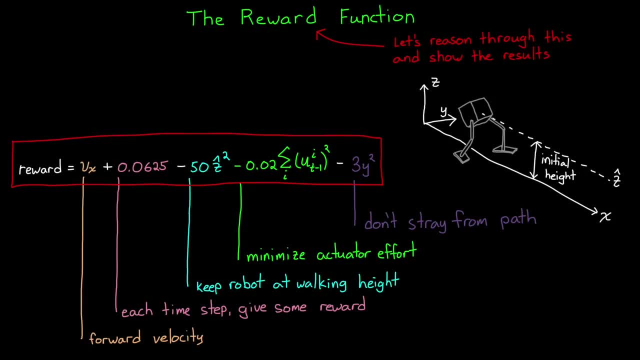 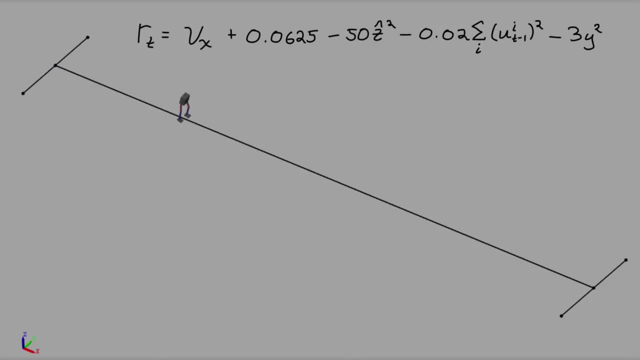 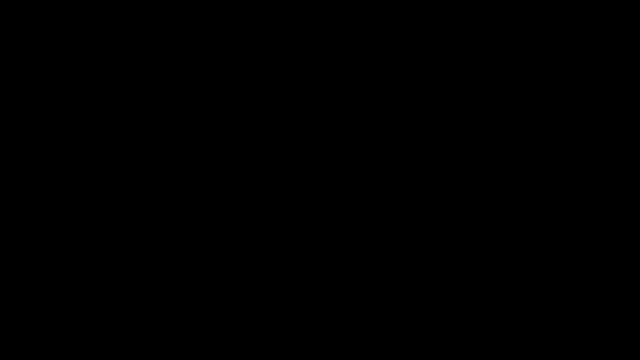 or a GPU or on a cluster of computers, then, after a few hours of training, we're going to have a solution. We'll have a robot that walks in a straight line in a human-like way. Let's move on to the policy. I've already stated that the policy is an actor neural network. 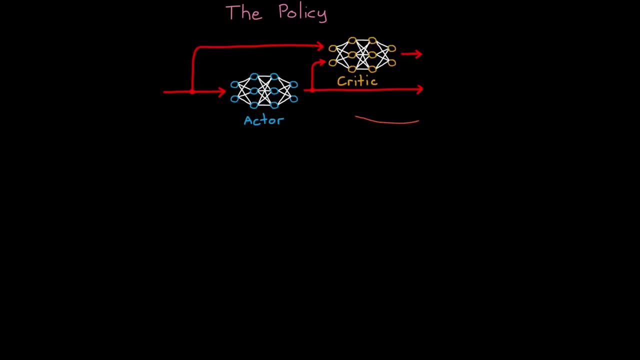 and along with it is a critic neural network, And each of these networks have several hidden layers of hundreds of neurons each, so there's a lot of calculations that go into them. If we don't have enough neurons, then the network will never be able to mimic the 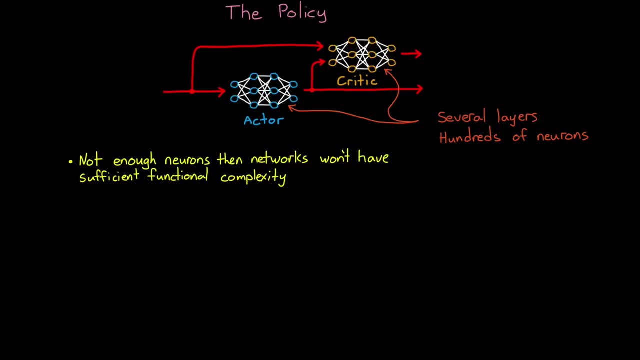 high-dimensional function that is required to map the 31 observations to the six actions for this non-linear environment. On the other hand, too many neurons and we spend more time training the excessive logic. In addition, the architecture of the network is really important. 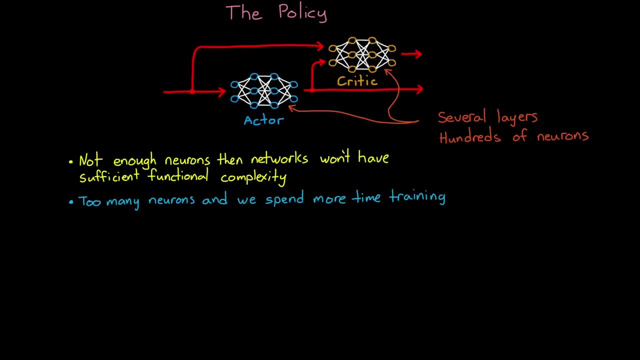 in functional complexity. These are things like the number of layers and how they're connected and the number of neurons in each layer. So there is some experience and knowledge needed to find that sweet spot that makes training possible and efficient, Luckily, as we know. 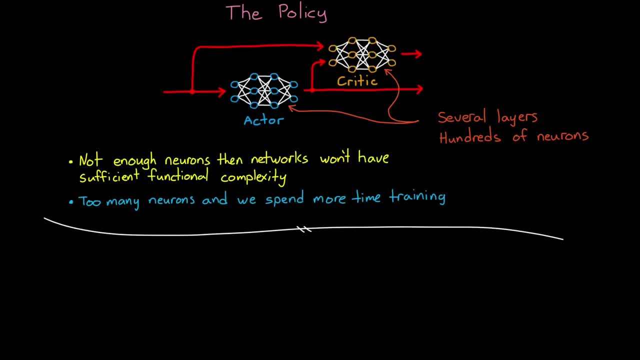 we don't need to manually solve for the hundreds of thousands of weights and biases in our networks. We let the training algorithm do that for us. In this example, we're using an actor-critic training algorithm called the Deep Deterministic Policy Gradient, or DDPG. 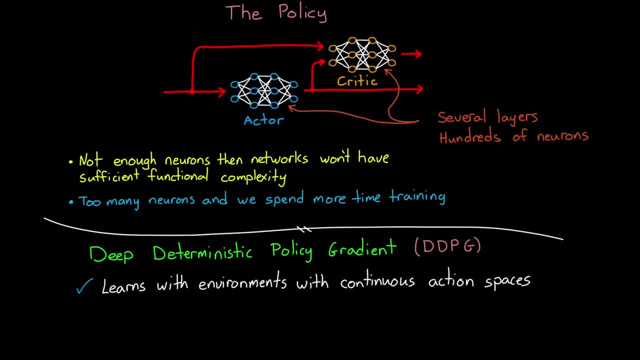 The reason is because this algorithm can learn with environments with continuous action spaces, like we have with the continuous range of torques that we can apply to the motors. Also, since it estimates a deterministic policy, it's much faster to learn than one that learns a. 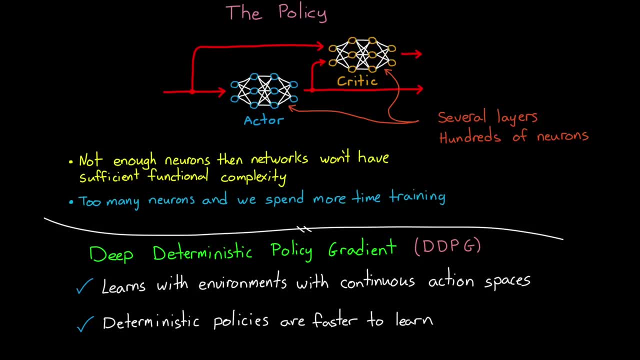 stochastic policy. I know this all sounds fairly complicated and abstract, but the cool thing to me about this is that most of the computer science that we use is based on the fact that the complexity is there for training the policy. Once we have a fully trained agent, then all we 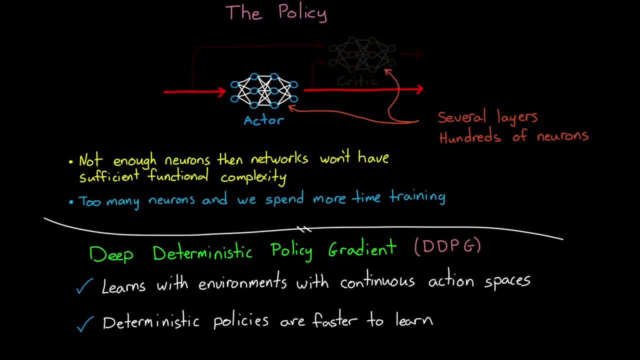 have to do is deploy the actor network to the target hardware. Remember, the actor is the function that maps observations to actions. It's the thing that's deciding what to do. It's the policy. The critic and the learning algorithms are just there to help determine the parameters. 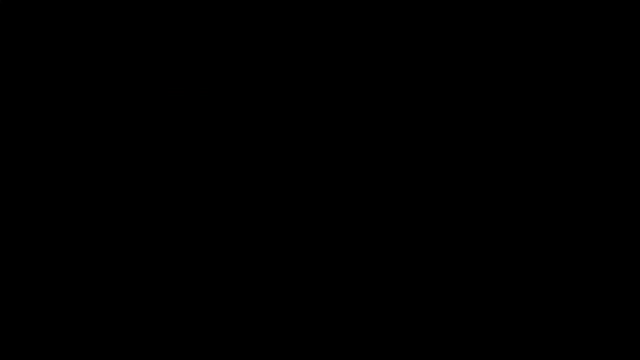 in the actor. Okay, at this point, here's a question that you might have. Sure, we can use RL to get a robot to walk in a straight line. However, won't this policy do only this one thing, For instance? 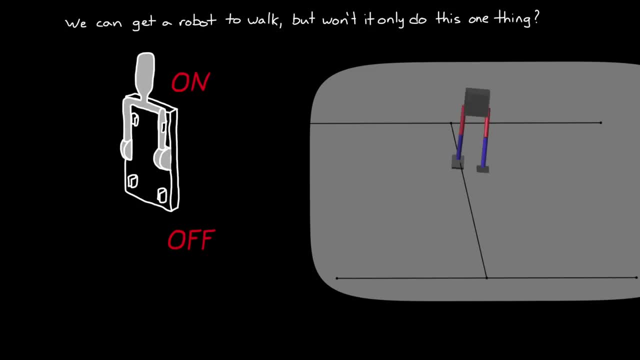 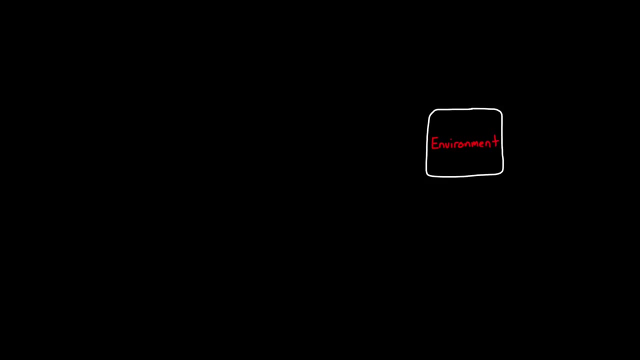 if I deploy this policy and turn on my robot, it's just going to instantly start walking straight forever. So how can I learn a policy that will let me send commands to the robot to walk where I want it to walk? Well, let's think about that Right now. this is what our system looks like. We 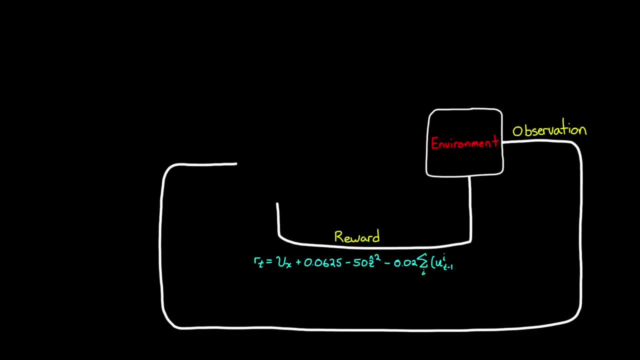 have the environment that generates the observations and the reward, and then we have the agent that generates the action. We have the environment that generates the observations and the reward, and then we have the agent that generates the action. Now, this is what our system looks like: We have the environment that generates the observations and the reward, and then we have the agent that generates the action. 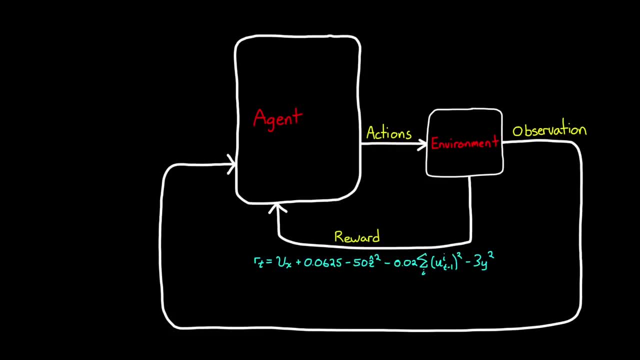 There's no way for us to inject any outside commands into this system and there's no way for our agent to respond to them, even if we had them, So we need to write some additional logic outside of the agent that receives a reference signal and calculates an error term. The error is the difference between: 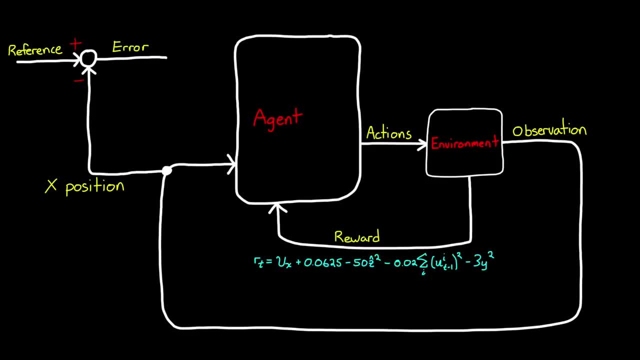 the current x position which we can get from the environment and the reference value. This is the same error calculation that we would have in a normal feedback control system. Now, rather than reward the agent for a higher velocity in the x direction, we can reward it for low error. This 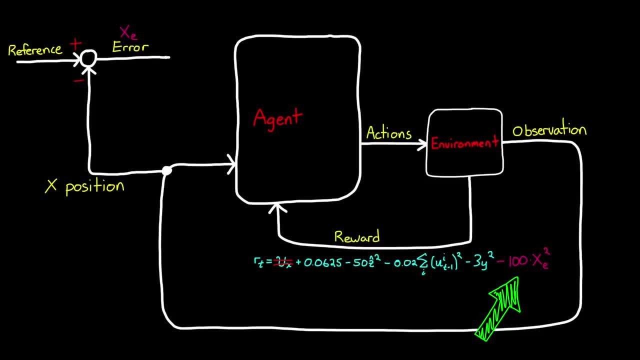 should incentivize the robot to walk towards and stay at the commanded x reference value For the observations. we need to give the agent a way to view the error term so that it can develop a policy accordingly, Since it might help our agent to have access to the rate of change of error and. 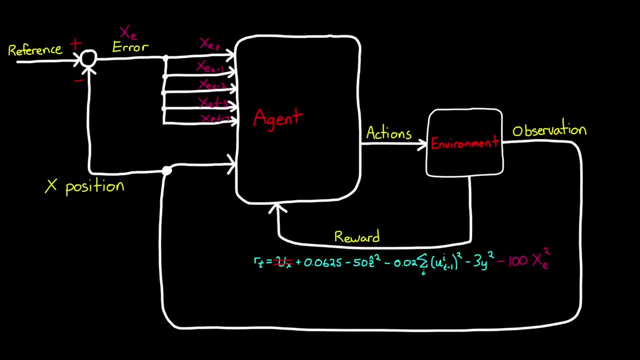 maybe other higher derivatives. I'll feed in the error from the last five sample times. This will allow the policy to create derivatives if it needs to. Eventually, the policy will be to walk forward at some specified rate if the error is positive and then backwards if it's negative. 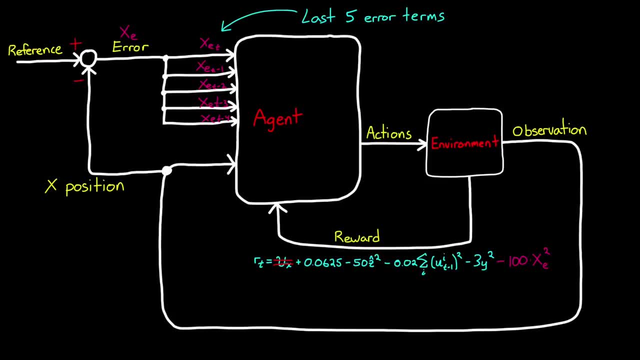 And since we now have 36 observations into our agent, we need to adjust our Actor Network to handle the additional inputs. Again, check out Sebastian's video in the description. if you need guidance on how to make changes, I've updated the default model in Simulink. 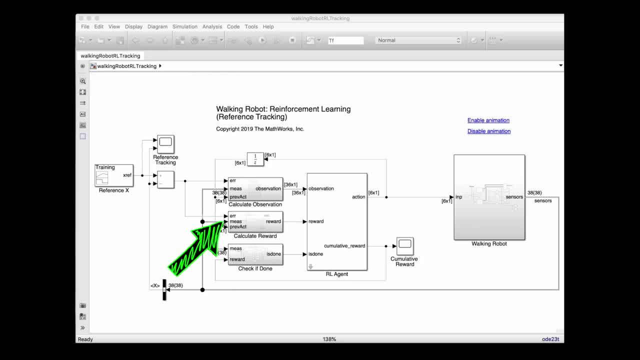 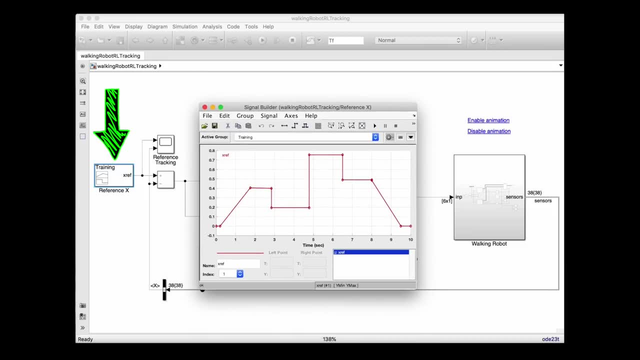 with the new Error term and fed it into the Observation Block and the Reward Block trained this agent over thousands of episodes using this particular profile, so it should be really good at following this profile. But the hope is that the trained policy will be robust enough to follow other profiles as well that have similar rates and accelerations. 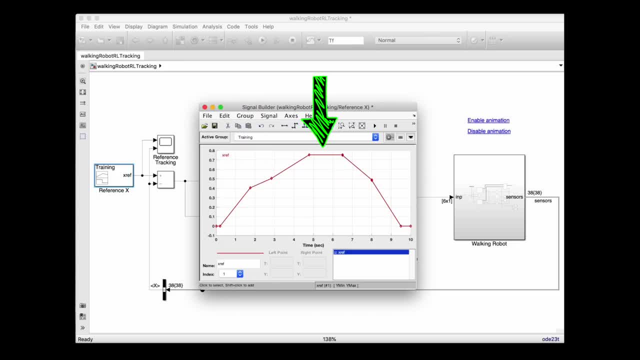 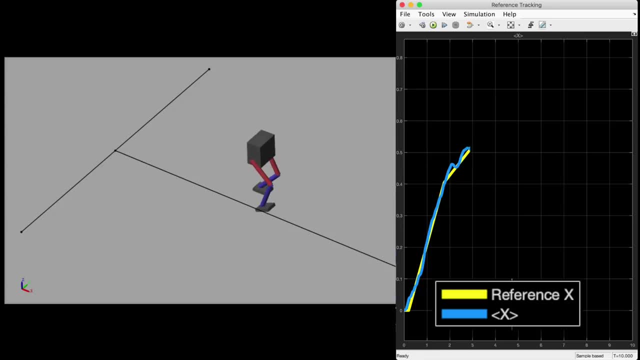 So let's give this a shot. I'll have it walk forward and then pause for a bit and then walk backwards. Okay, it's kind of funny looking when it walks backwards. but overall, a pretty good effort, With some reward tweaking and maybe a little more time spent training. I might be on to. 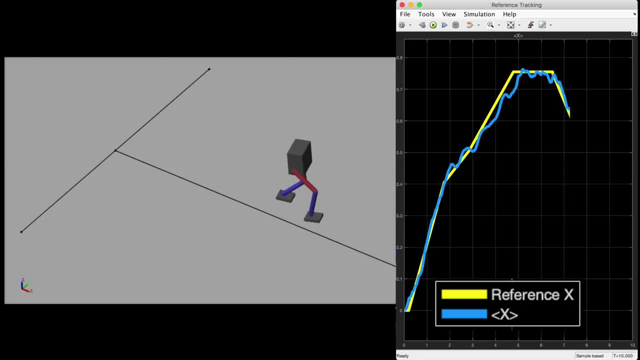 something pretty good here. So in this way you can start to see how we can use an RLAgent to replace part of the control system. Instead of a function that learns a single behavior, we can extract the high-level reference signal and have the agent work off error, so that 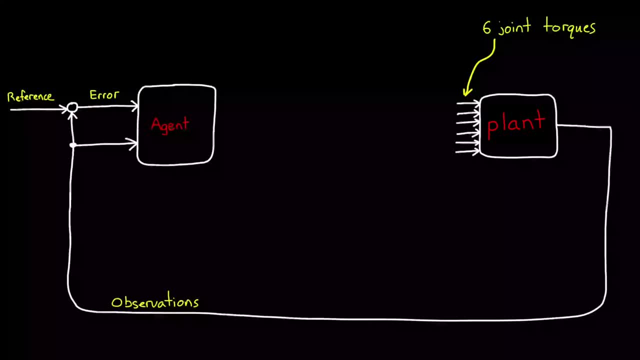 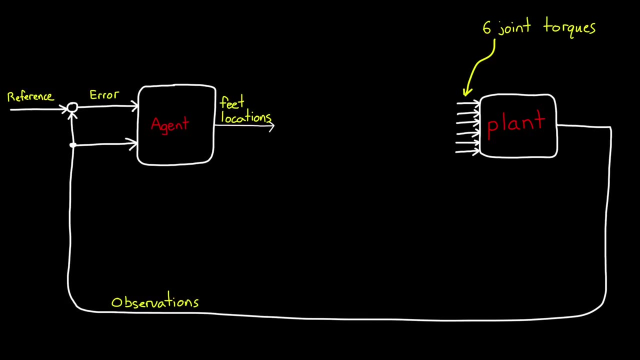 we can retain the ability to send commands. We can also remove low-level functionality from the agent. For example, instead of the actions being the low-level torques for each of the six joints, the agent could just learn where to place its feet on the ground, So the action would be place left foot at some. 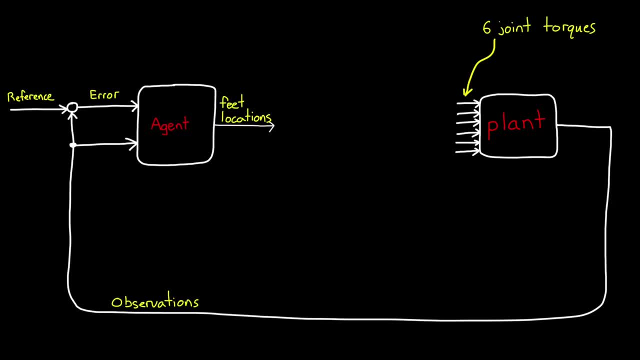 location in the body coordinate frame. This action could be the reference command for a lower-level traditional control system that drives the joint motors. You know something that might feed forward a torque command based on your knowledge of the dynamics of the system and the control system. 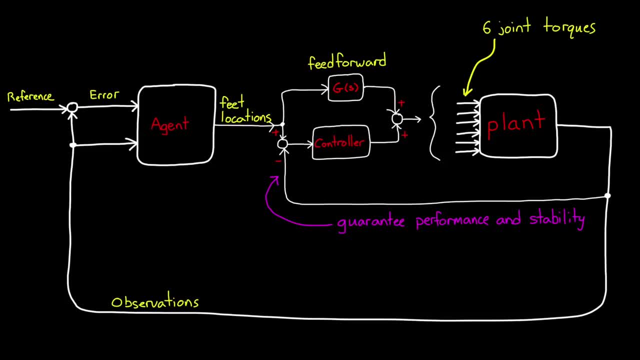 And then feed back some signal to guarantee performance and stability. And this is beneficial because we can use our specific domain knowledge to solve the easy problems And that's going to give us insight and control over the design. And then we can reserve reinforcement learning for the problems that are more difficult. 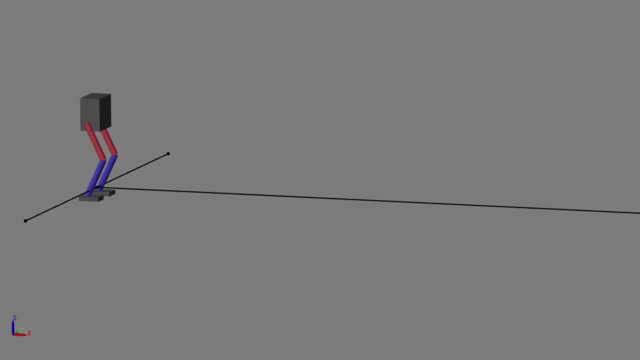 Something to note about our final walking solution is that it's really only robust to its own state. You know. it can walk around without falling over, which is good, but only in a perfectly flat feature. It's not taking into account any part of the world outside of the robot, so it's actually 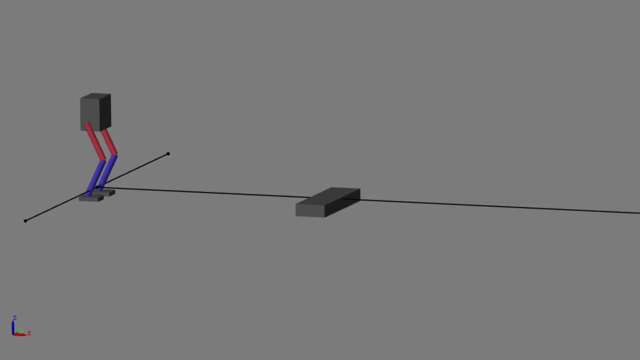 quite a fragile design. For example, let's see what happens if we place a single obstacle in the way of our robot. Well, that went pretty much as expected. The problem here is that we didn't give our agent any way of recognizing the state of the environment beyond the motions of the robot itself. There's